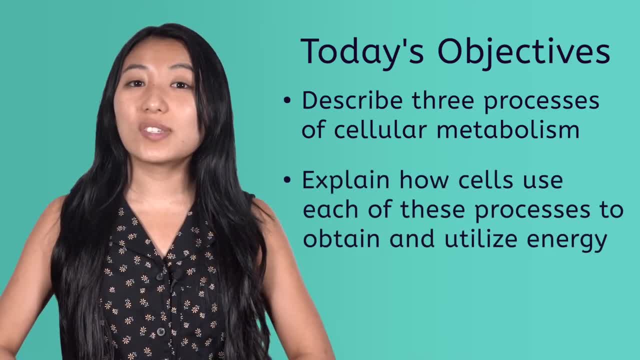 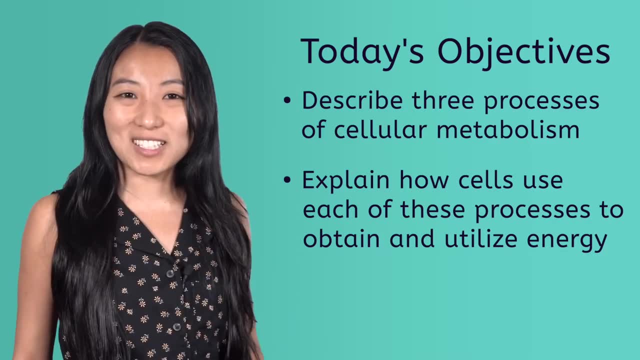 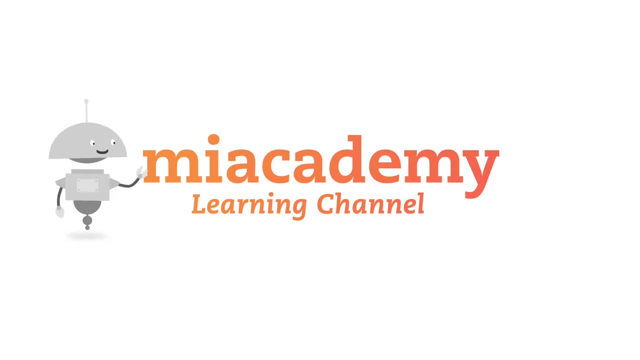 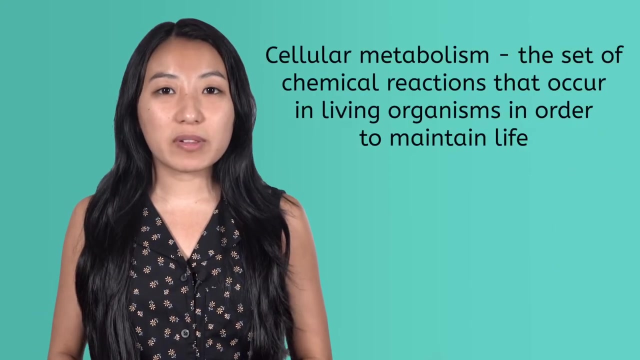 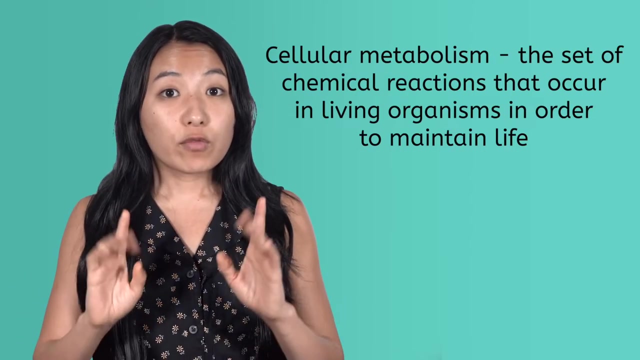 metabolism and explain how cells use each of these processes to produce energy. Let's get into it. Cellular metabolism is the set of chemical reactions that occur in living organisms in order to maintain life, Remember, our bodies strive for homeostasis or balance, and so 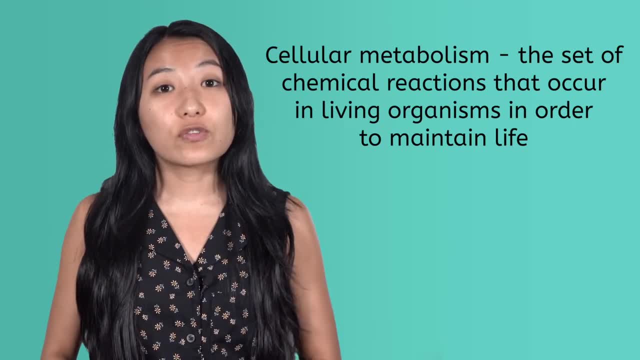 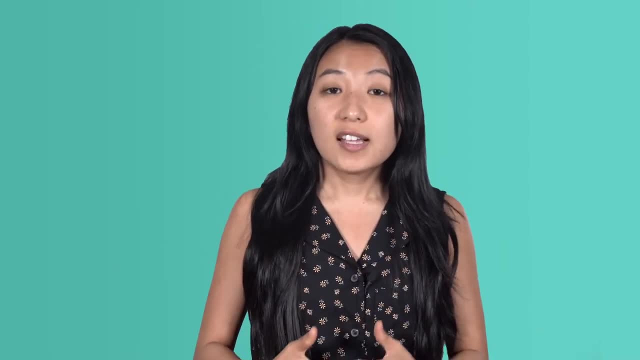 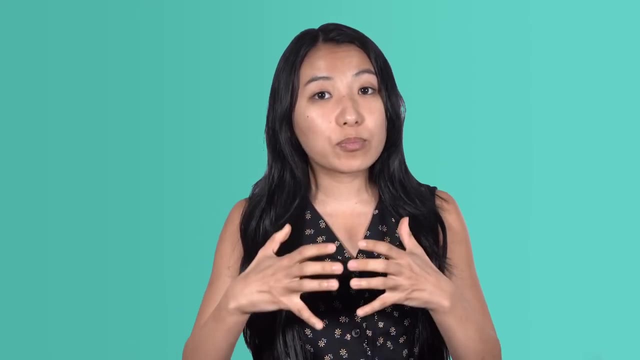 cellular metabolism, like cellular transport, is essential for maintaining this balance. While cellular transport deals with moving resources in and out of cells, cellular metabolism involves reactions that chemically change these resources, allowing cells to capture and store energy that is essential for their survival. 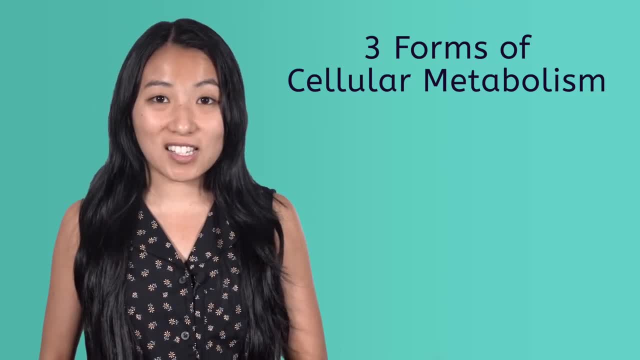 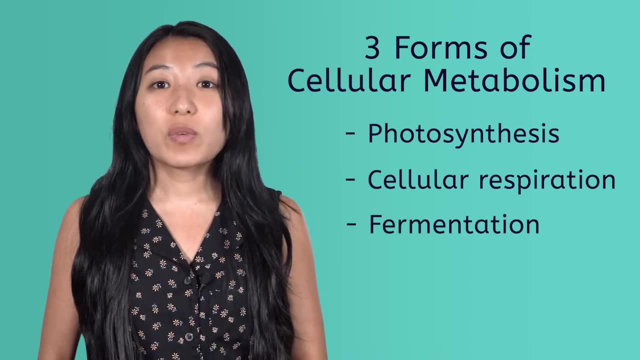 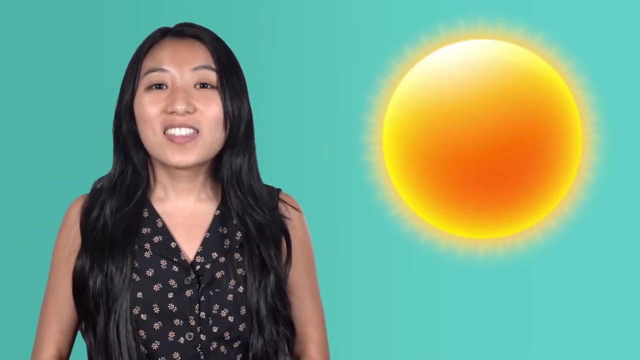 There are three main forms of cellular metabolism we will discuss today, and they are photosynthesis, cellular respiration and fermentation. To understand how energy flows through living things, we have to start with the source: the sun. The sun provides all of the energy needed to sustain life on Earth. Sunlight enables 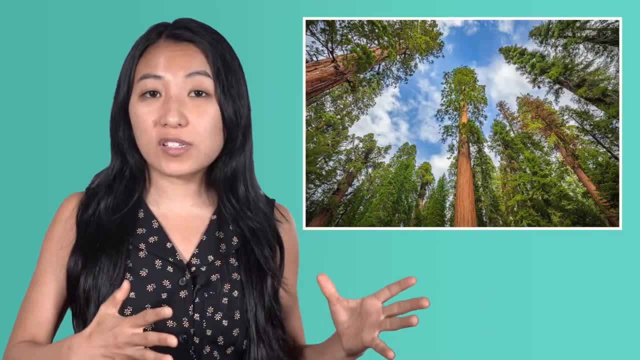 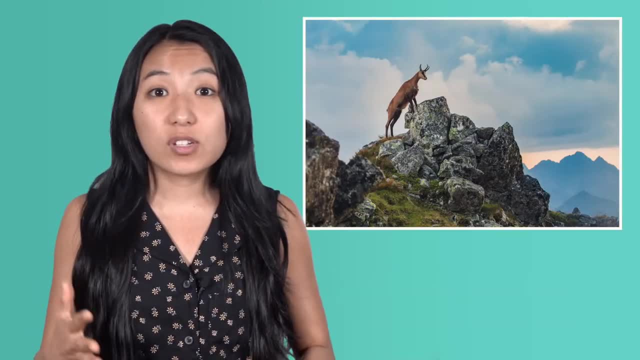 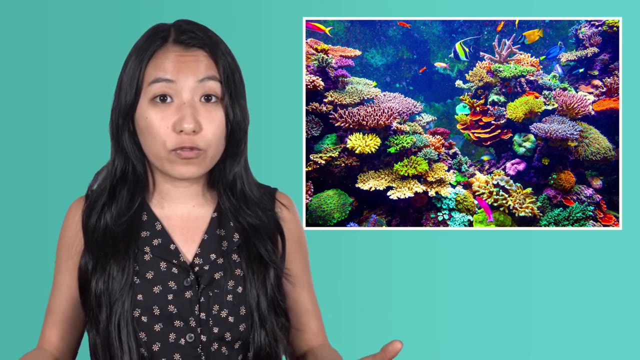 the growth of vast jungles, towering redwood forests and sprawling grasslands, supporting life in countless ecosystems, including deserts, mountains, marshes and tundras. It permeates our oceans, filtering energy into massive kelp forests and coral reefs, which, in turn, 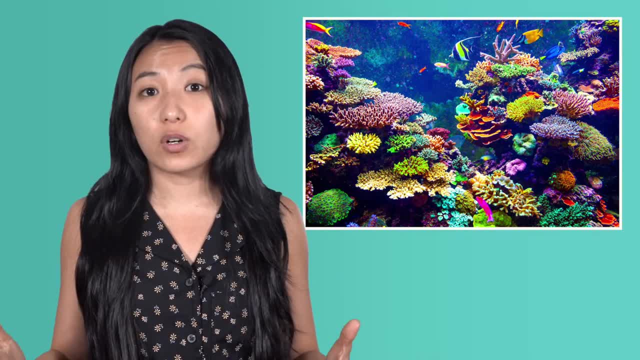 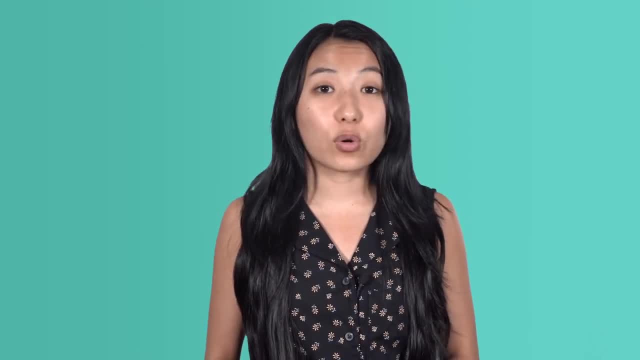 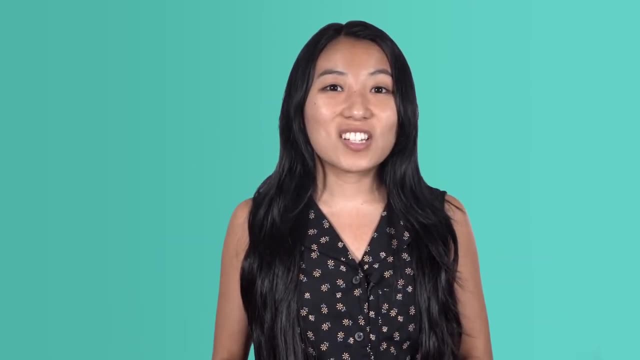 provide food and sanctuary for many other living organisms. So if sunlight is the original source of energy, how do plants and other organisms capture the sun's energy to make Earth's rich ecosystems possible? The sun's energy is captured in a process called photosynthesis, which is a series of reactions occurring in 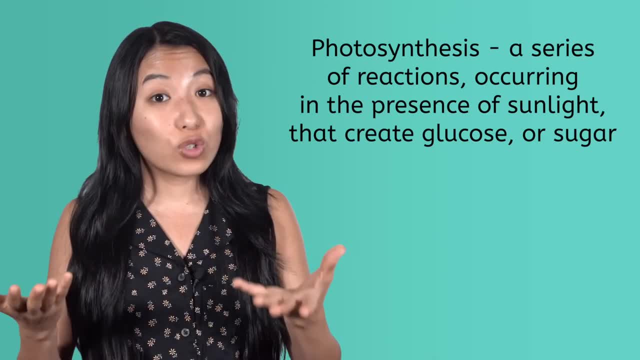 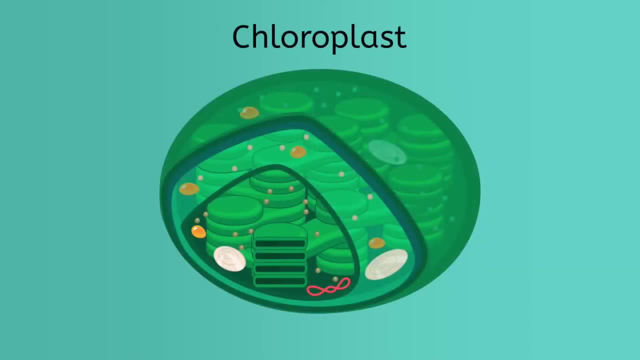 the presence of sunlight that create glucose or sugar. Photosynthesis occurs in specialized organelles called chloroplasts, which can only be found in some organisms such as plants, algae and special types of bacteria. The green color of this organelle, and consequently most plants, comes from the pigment chlorophyll. 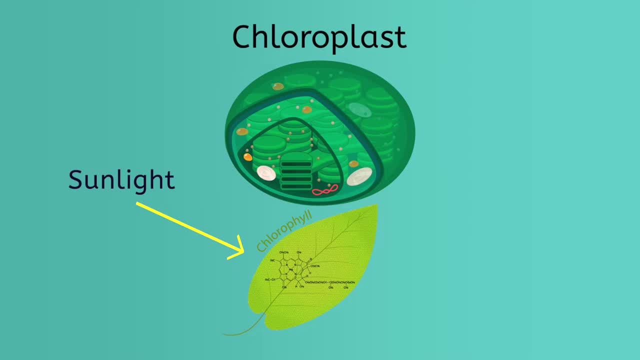 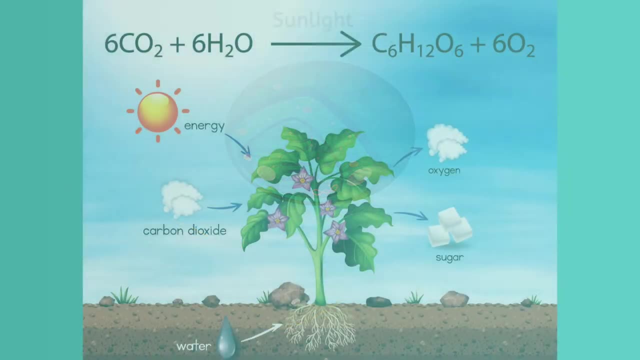 which is used to absorb the energy from sunlight. Once light energy is absorbed, it sets off a chain of reactions that is summarized by this equation: 6 CO2 plus 6 H2O plus sunlight yields C6H12O6 plus 6 O2.. 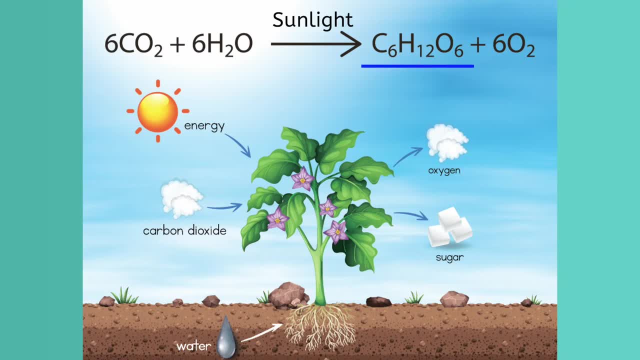 C6H12O6 is the chemical formula for glucose or sugar, which has 6 carbon atoms, 12 hydrogen atoms and 6 oxygen atoms. Notice anything about our equation. If you count up all the carbon, hydrogens and oxygens on each side, they match. 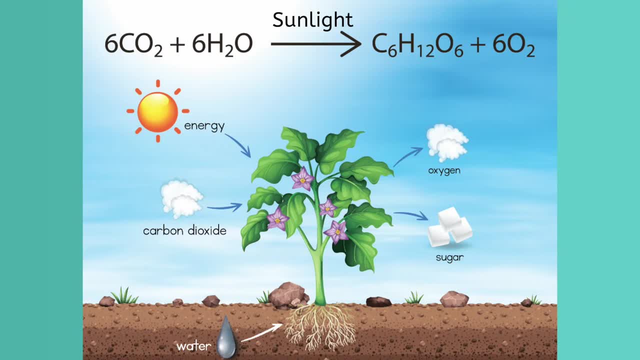 Plants can't create glucose- nature's miracle food- out of nothing. The word photosynthesis comes from the words photo, meaning light, and synthesis, which means put together. Plants and other photosynthesizing organisms use chemical reactions to put together glucose. 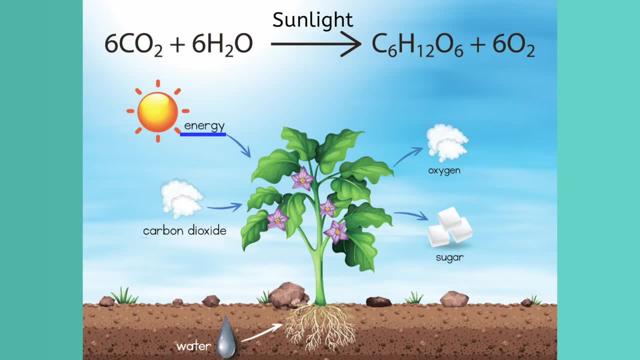 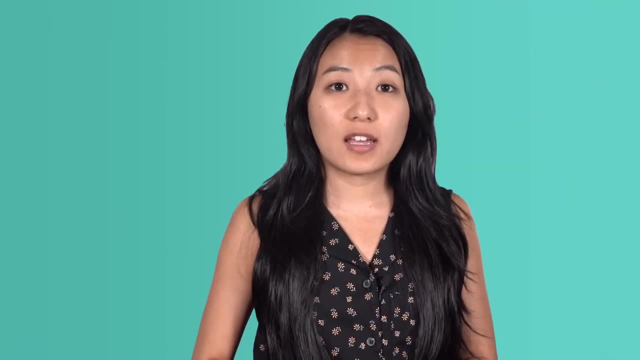 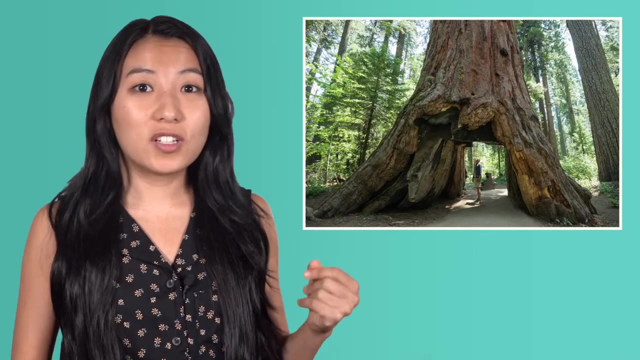 or sugar, using water, carbon dioxide and energy from sunlight, while producing oxygen as a waste product. Plants use the glucose they make in a variety of ways, but the main purpose is to help them grow. All plants on Earth, even this mighty redwood, start from humble beginnings such as seeds. 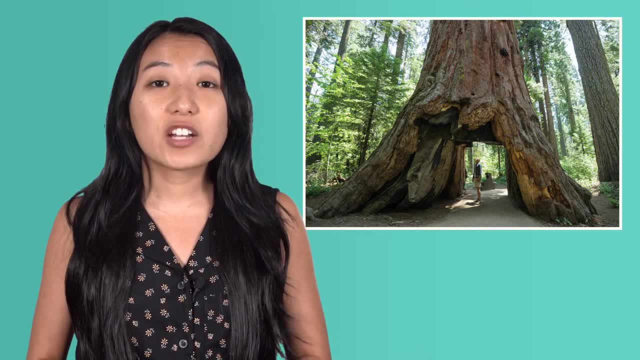 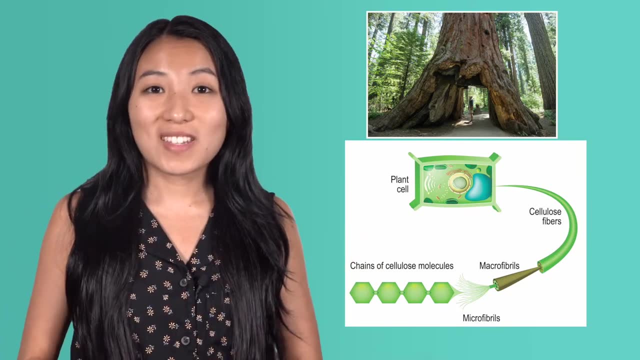 or spores, and build themselves over time out of a starch called cellulose, which is basically a ton of glucose chained together. Plants also use glucose to build additional sugars, starches and fats. They have a lot of glucose in them, but they're not all the same. 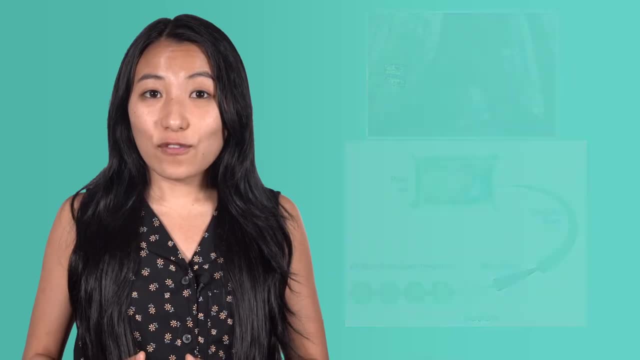 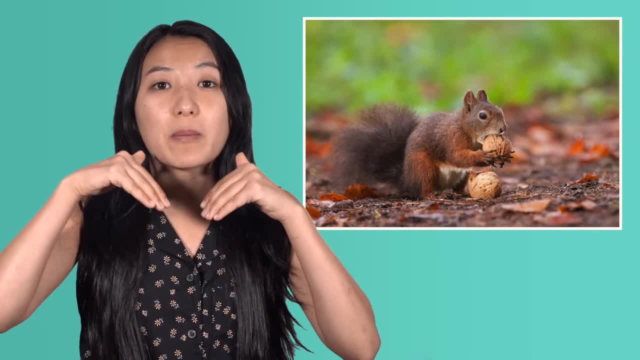 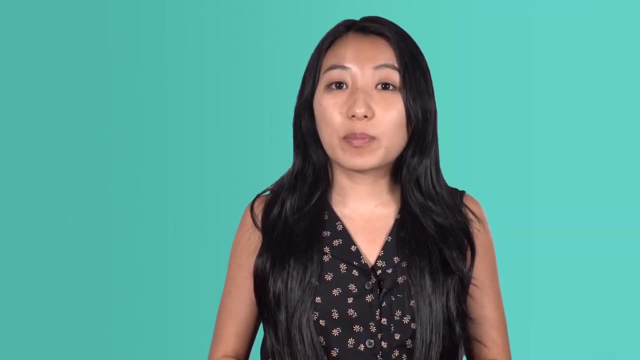 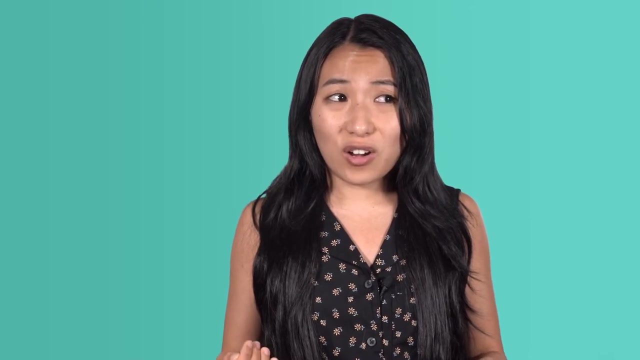 Plant-eating organisms then eat these resources, breaking them back down into glucose, giving rise to massive food webs. This glucose is relied upon for food by almost every living thing that can't photosynthesize, so it's hard to overstate the importance of this process. 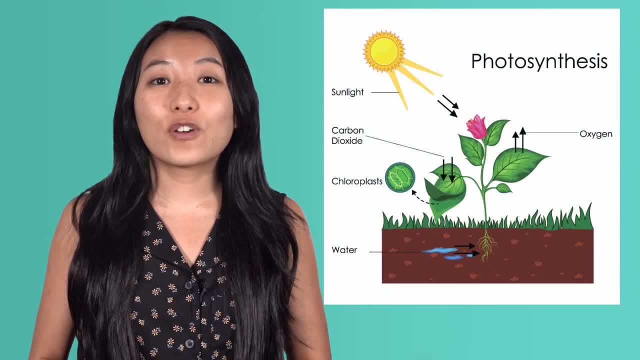 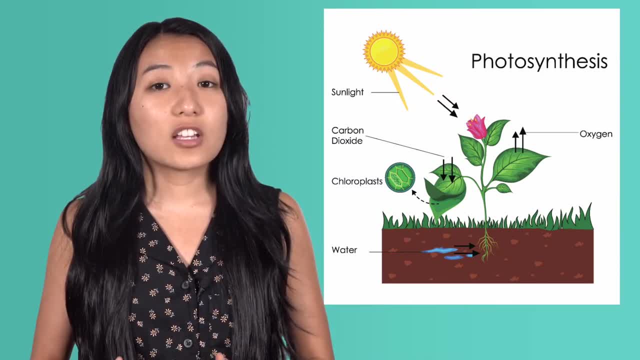 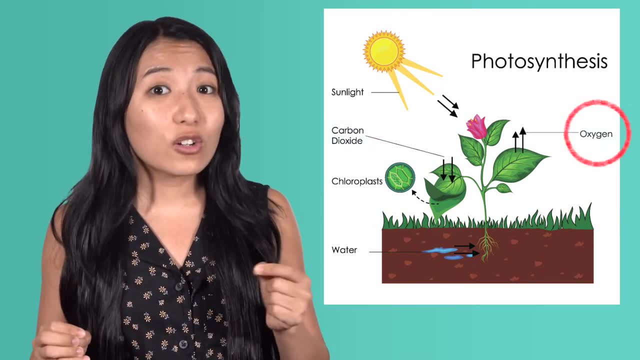 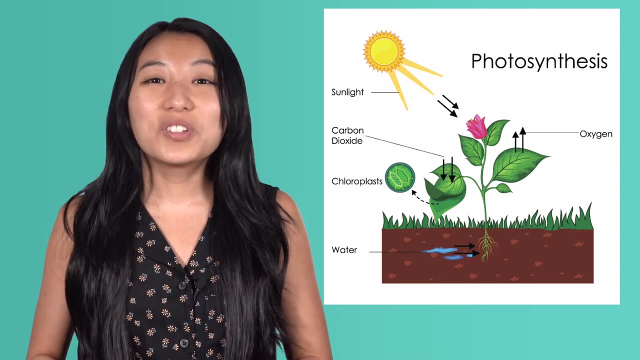 how much carbon in the atmosphere by taking carbon dioxide out the air and replacing it with oxygen gas, which is a vital resource for many living things. In order to understand just how important oxygen is, we'll need to talk about a process called cellular respiration. 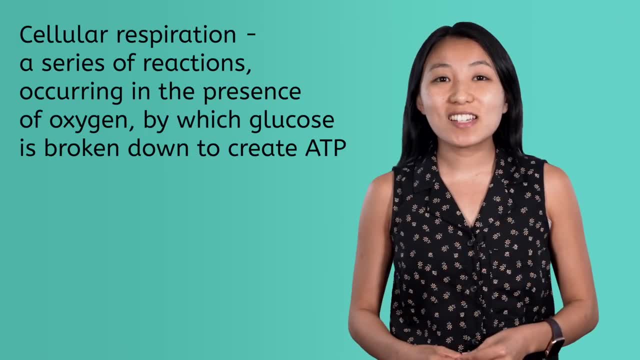 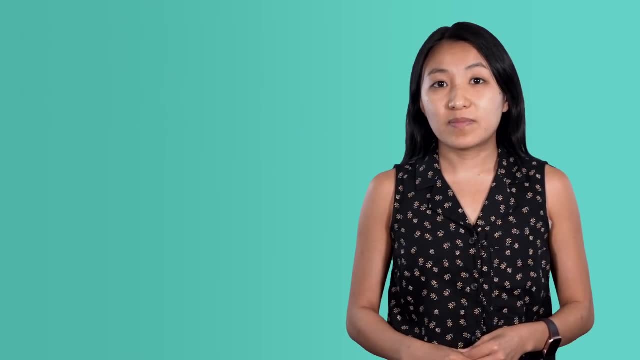 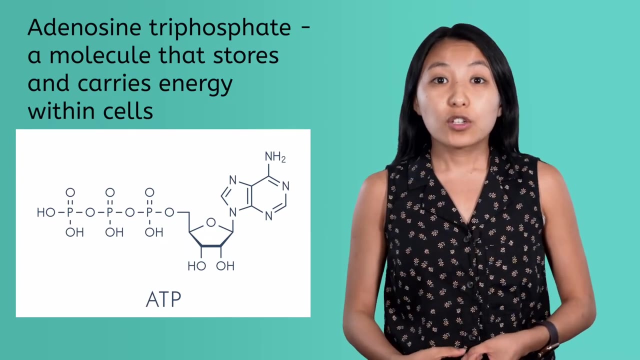 Respiratory Universe. Cellular respiration is a series of reactions occurring in the presence of oxygen, by which glucose is broken down to create ATP. ATP, or adenosine triphosphate, is a molecule that stores and carries energy within cells. Your cells are constantly spending ATP to survive, and cellular respiration is their 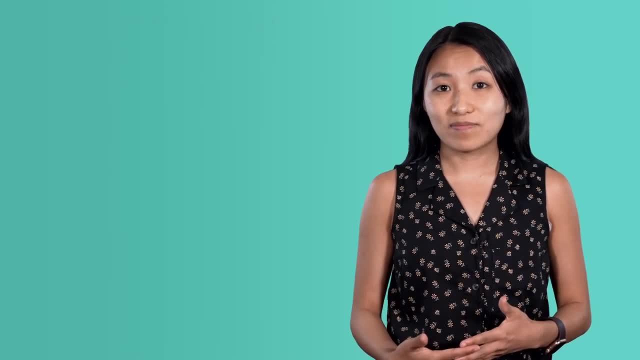 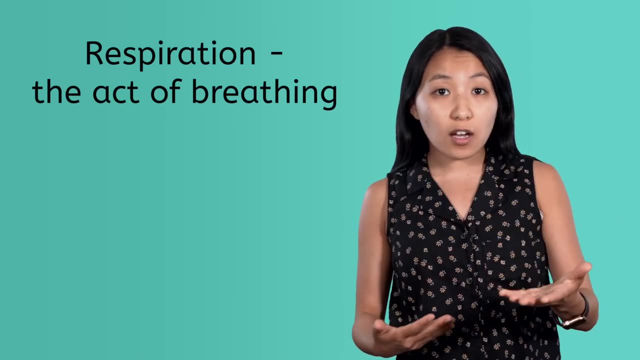 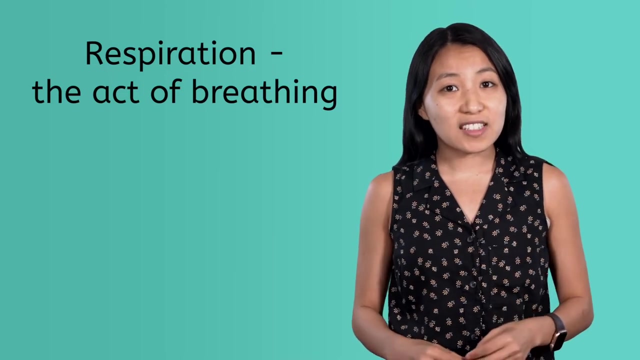 way of replenishing it so they don't run out. The term respiration means the act of breathing, so you can think of cellular respiration as breathing at a cellular level. It is important to understand that it is our individual cells that need oxygen, gas specifically. 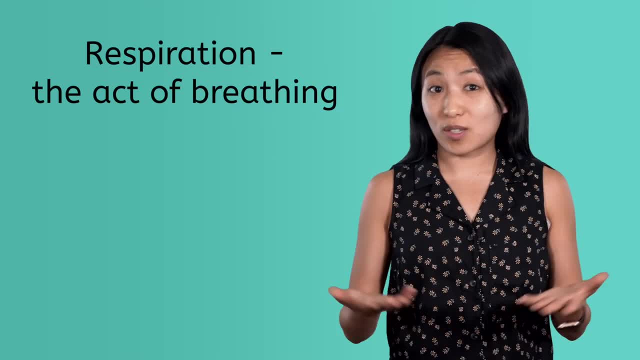 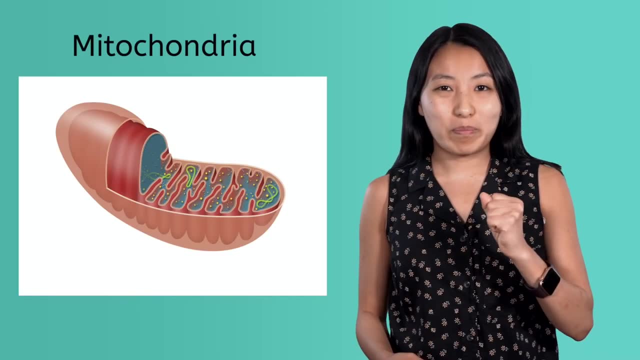 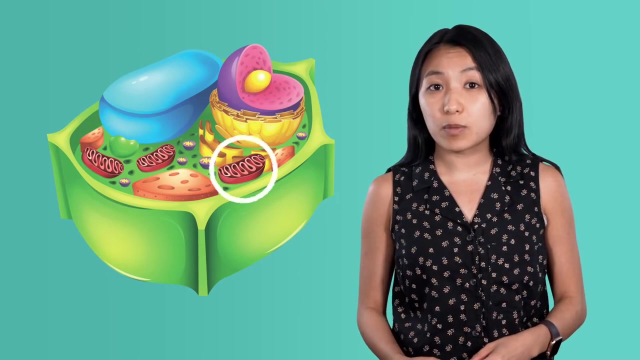 for this process of creating ATP, which is why we breathe at all. Cellular respiration occurs in the mitochondria, or pituitary gland, Powerhouse of the cell. It's worth noting that plants have mitochondria and do, in fact, perform cellular respiration. 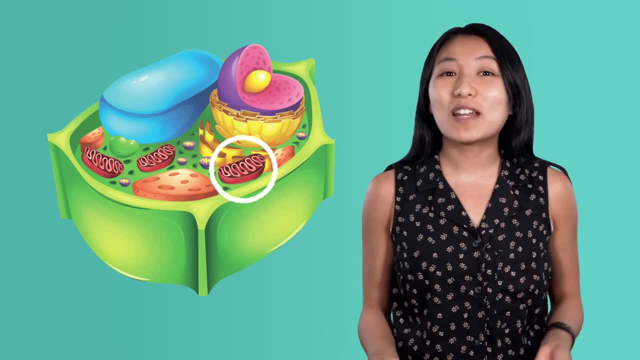 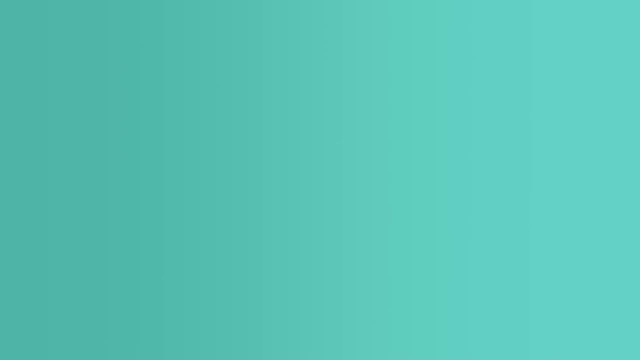 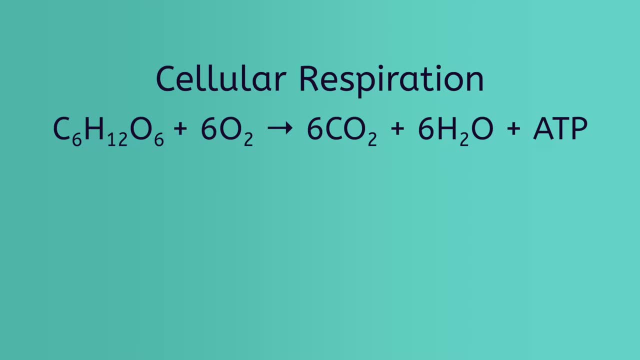 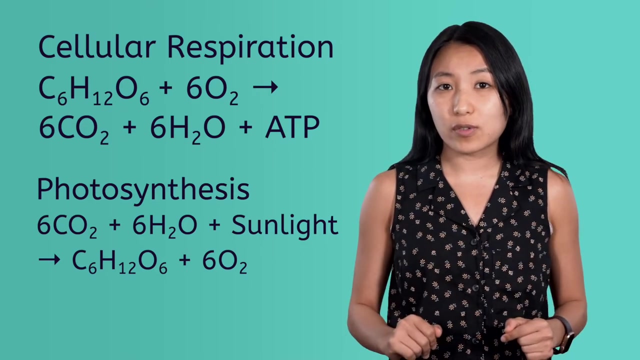 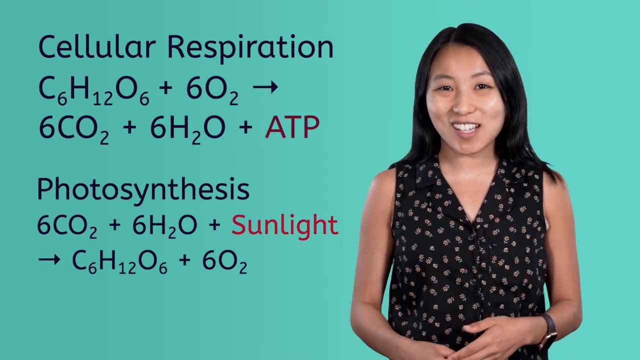 C6H12O2 yields 6CO2 plus 6H2O, plus ATP. Remember, C6H12O6 is glucose. As you might notice, this equation for cellular respiration is very similar to photosynthesis, just in reverse order and involving stored energy as ATP instead of sunlight. 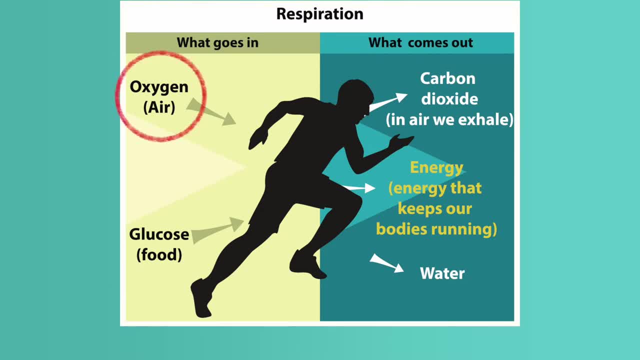 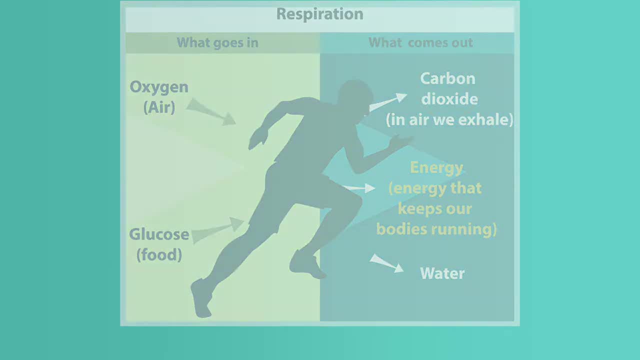 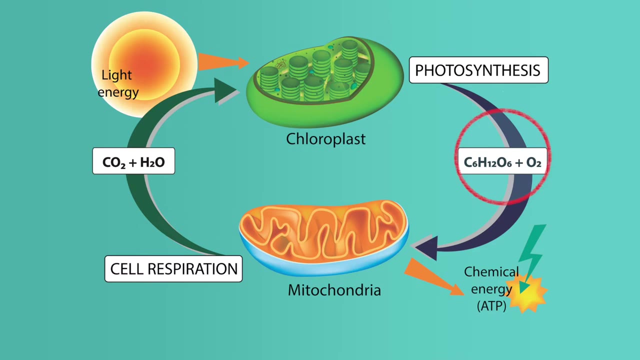 With this process, organisms breathe in oxygen and consume oxygen. They then consume glucose in order to produce stored energy, while expelling water and carbon dioxide as waste products. Carbon dioxide and water are then used by plants for photosynthesis to create glucose and oxygen, repeating the cycle. 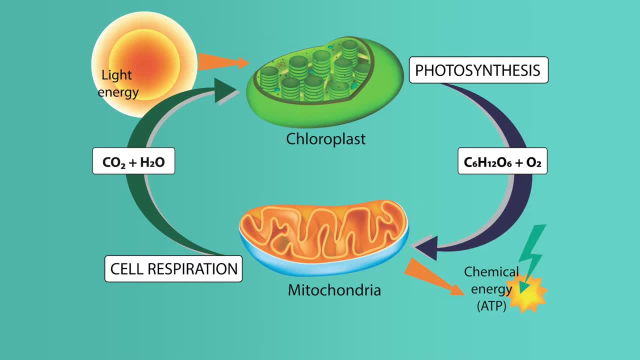 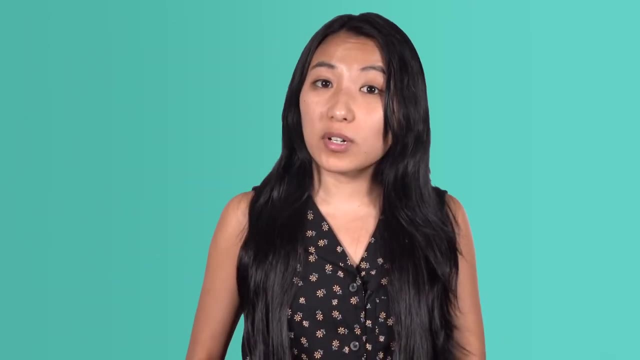 In this way, photosynthesis and cellular respiration complement each other, recycling each other's waste to maintain a healthy balance of resources on Earth, all while keeping energy flowing through living things. OK, we've now covered how organisms capture energy using oxygen. 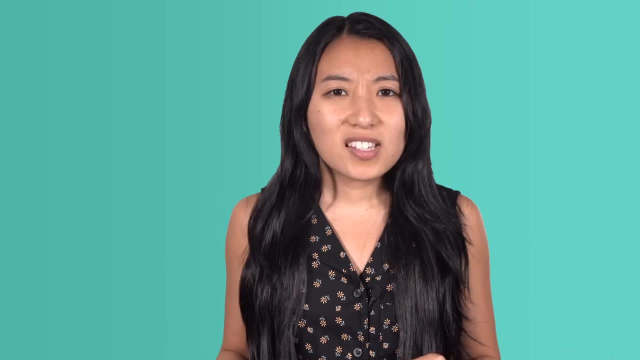 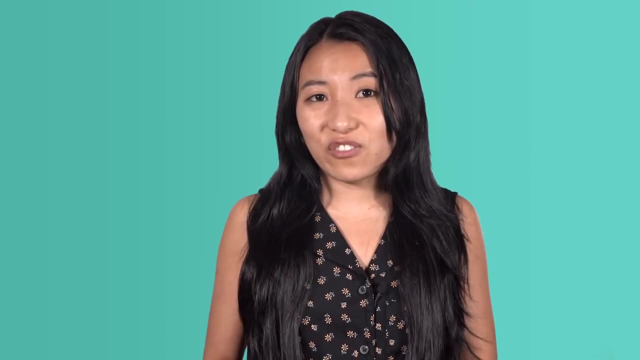 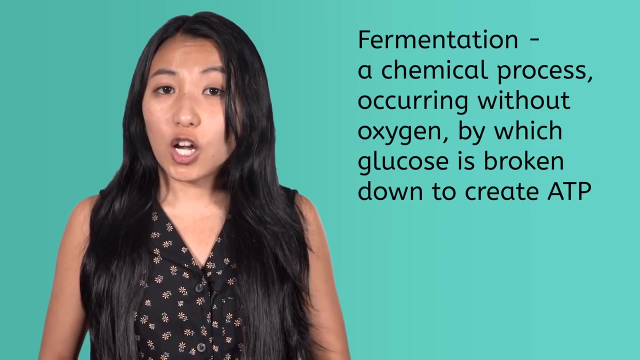 But what happens when oxygen isn't present? In this case, is it possible for cells to make any energy at all? Well, actually they can, but it is not nearly as efficient at creating ATP as cellular respiration. Fermentation is a chemical process occurring without oxygen, by which glucose is broken. 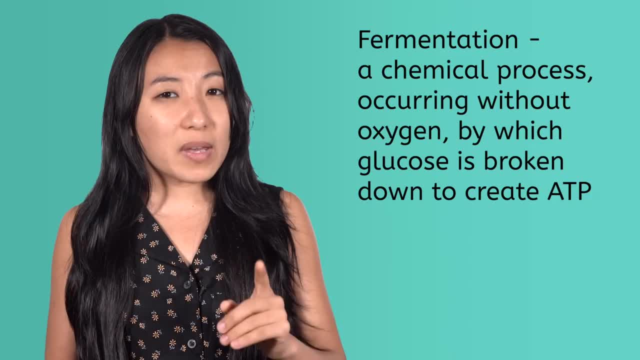 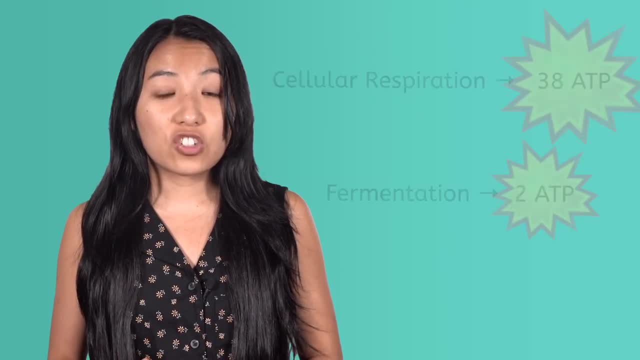 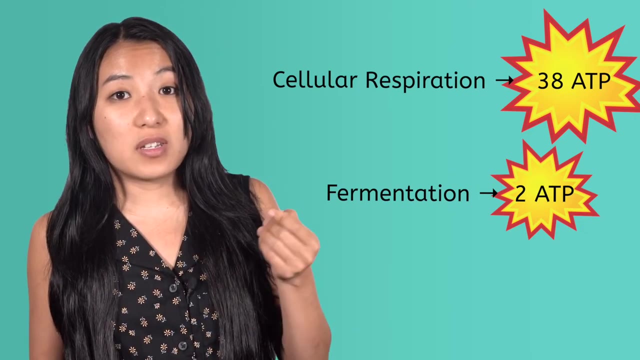 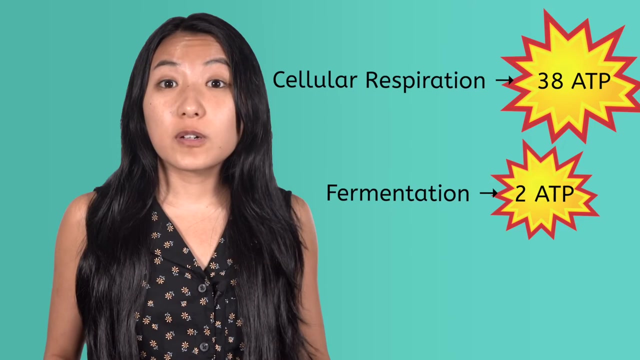 down to create ATP. The big difference between cellular respiration and fermentation is that one cycle of cellular respiration generates a whopping 38 ATP molecules, while fermentation only yields a measly two from the same amount of glucose. And to add insult to injury, fermentation creates byproducts like ethyl alcohol and lactic acid that clog up cells. So what happens? The type of byproduct depends on the type of fermentation. If you've ever exercised so hard that you struggled to breathe and felt that heavy, achy feeling in your muscles, you know what lactic acid feels like. 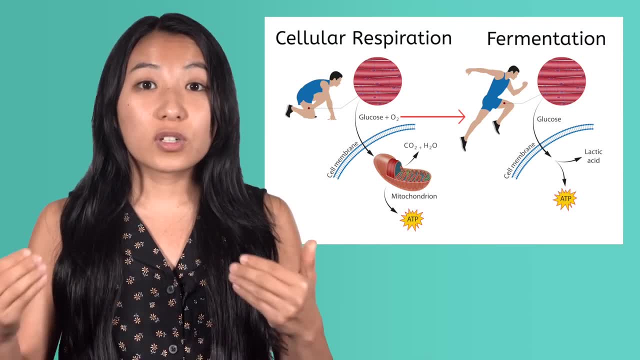 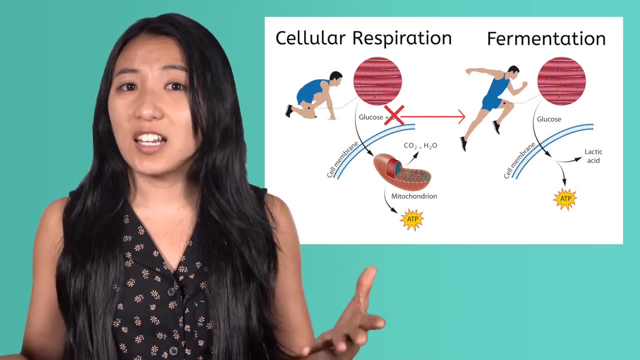 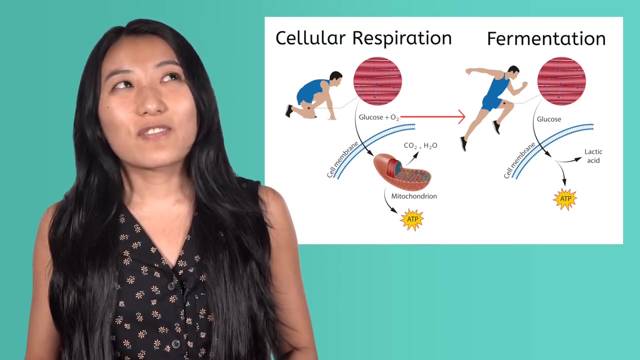 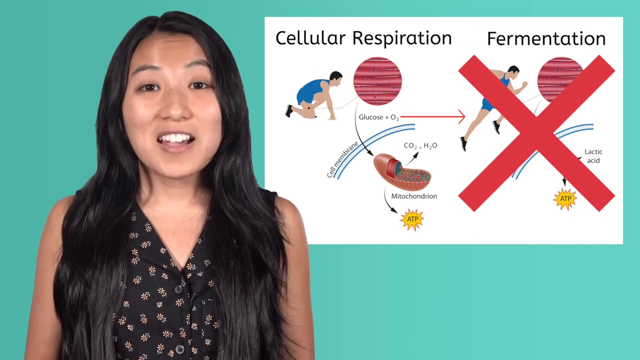 Your body performs lactic acid fermentation when your lungs can't keep up with the oxygen demands of your muscles or there simply isn't any oxygen present. It's good to know our bodies have a backup system in place, but fermentation is definitely not a good way for us to obtain energy in the long term. Plants and other organisms can use fermentation as well, but typically only do so when oxygen is scarce. However, some organisms ONLY use fermentation to generate ATP. Bacteria, for example, Bacteria such as Lactobacillus, survive by using lactic acid fermentation. 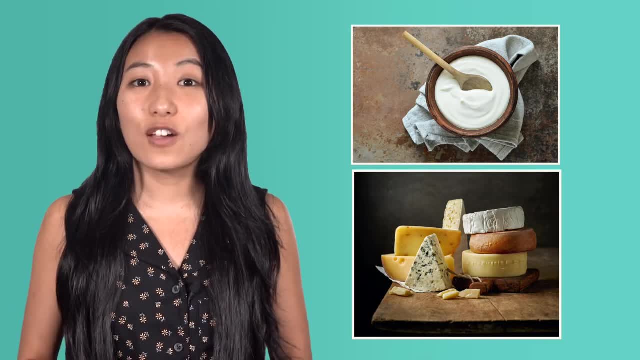 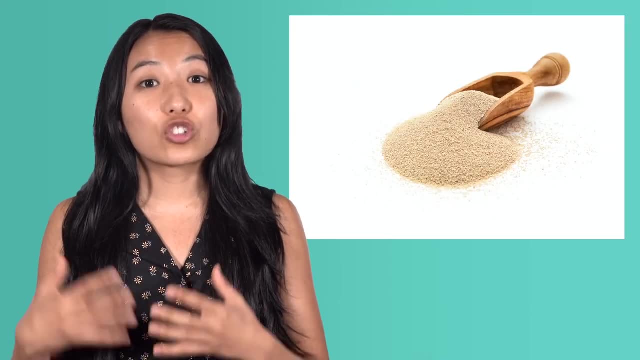 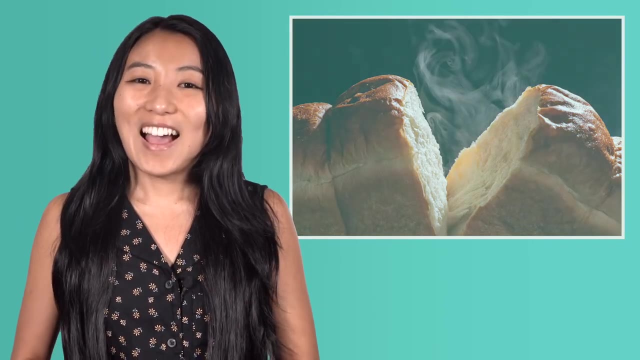 Yogurt and cheese are examples of food created from this fermentation process. Another example is yeast, which is a fungus that ferments sugars and is responsible for making bread rise or puff up when baked. As you can see, fermentation is important for a variety of organisms.